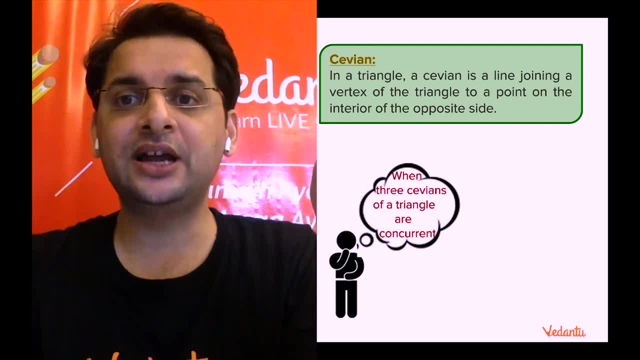 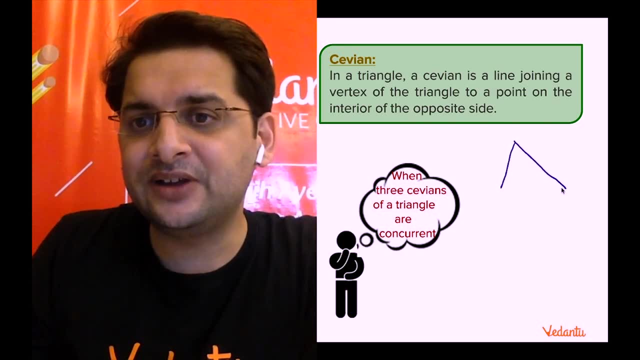 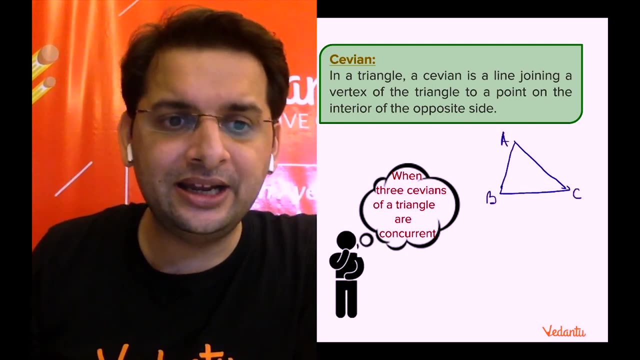 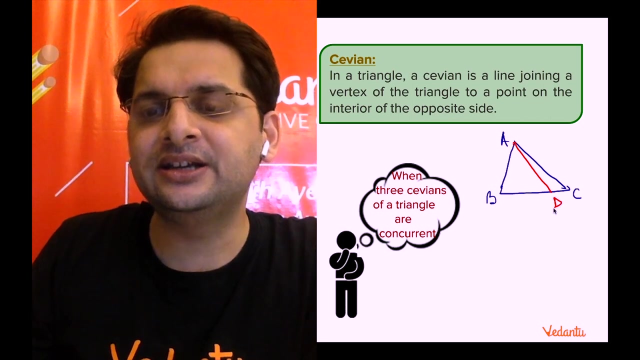 So in a triangle, a C1 is a line which joins a vertex of the triangle to the point on the interior of the opposite side. So let's say: if it is a triangle ABC, So if this is a triangle ABC, so any line joining the vertex A to any point on the opposite side, let's say this is D. 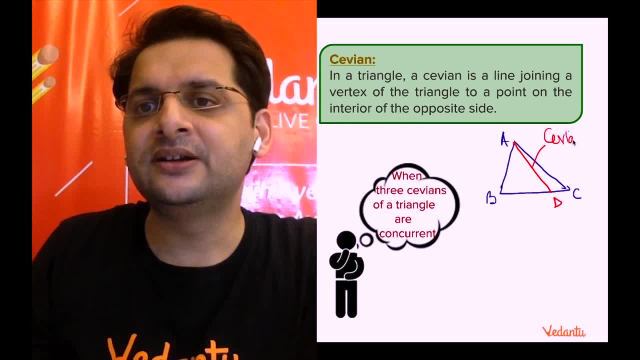 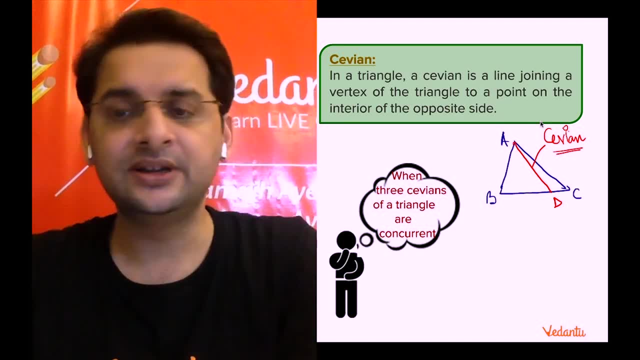 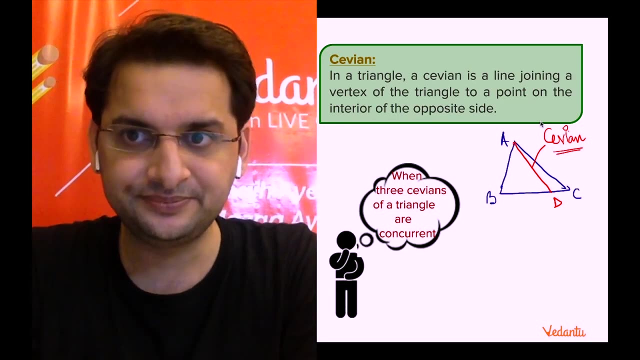 So this is called a C1.. This is called a C1.. So the theorem is related to a C1.. The theorem is related to a C1. So there are, ultimately, there are infinitely many C1s. which joins A to any point of BC. 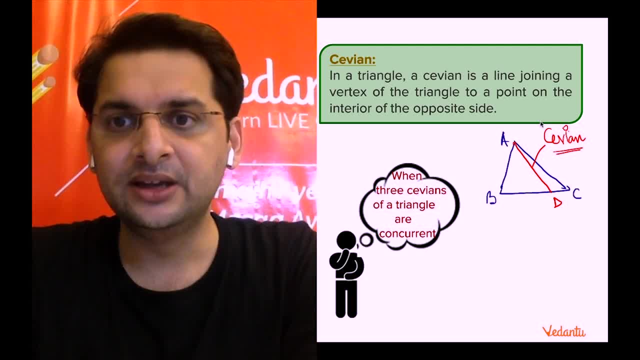 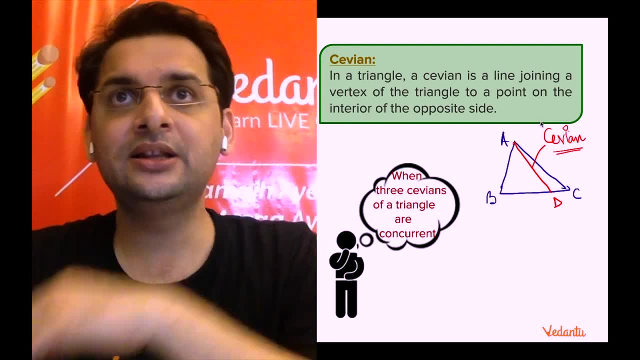 Ok, So in a triangle there are infinitely many C1s, So the median is one of the C1.. The angle bisector is one of the C1s. In an acute triangle, the altitude is one of the C1s. 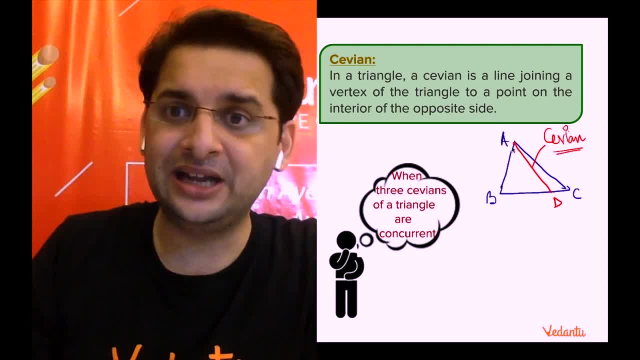 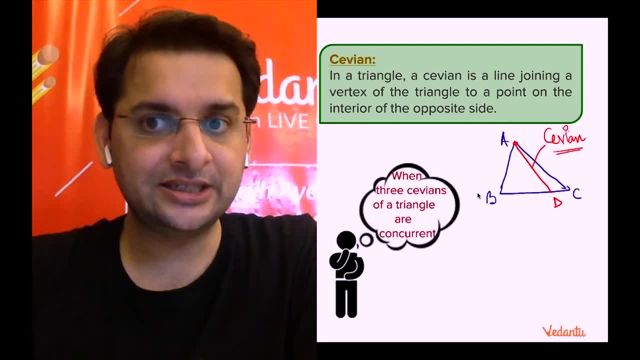 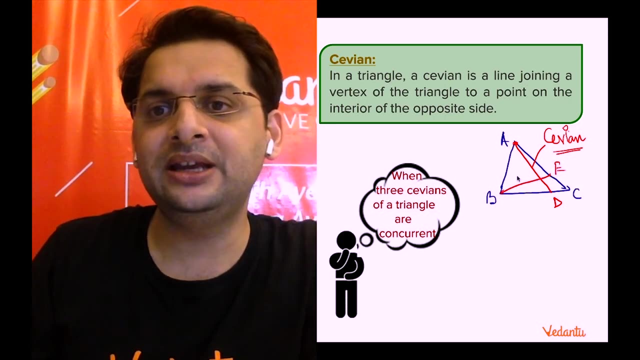 So there are infinitely many C1s. Ok, so there are plenty of lines which I can join from vertex say A to any point on BC, Right? so the question is, when are the three C1s? If there are three C wins, let's say A, D, B, E and let's say C, F, which passes to this point. 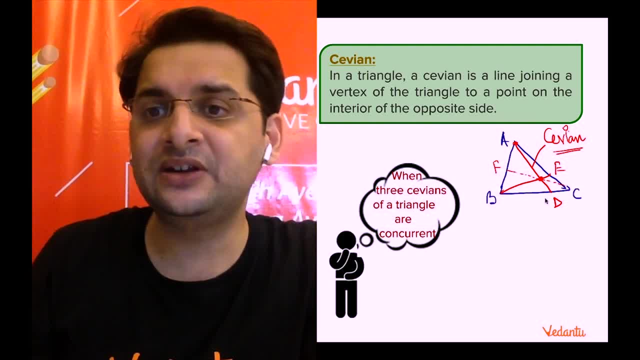 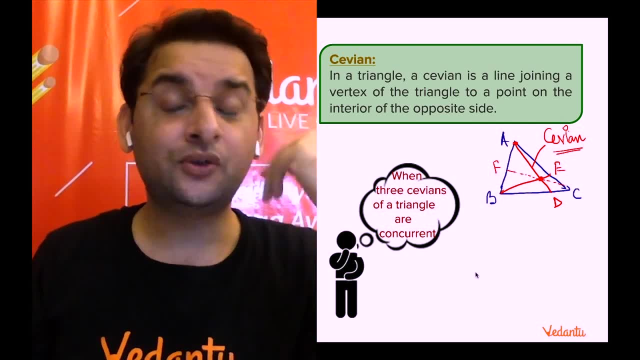 So what is the condition? that the three C wins from three different vertices of a triangle are concurrent. Concurrent means they meet at a common point. So what is the condition? What is that condition Right? So we'll be studying that condition via Siva's theorem. 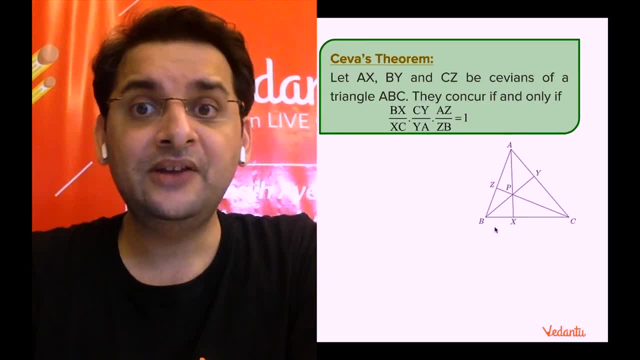 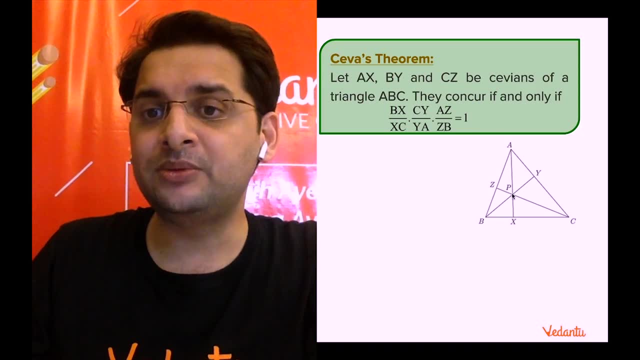 So what is Siva's theorem? Siva's theorem says: if AX and BY and CZ are three C wins of a triangle ABC, then they conquer. Conquer means they meet at a common point. only and only if BX, upon XC, into CY, upon AY, into AZ upon ZB, is equal to 1.. 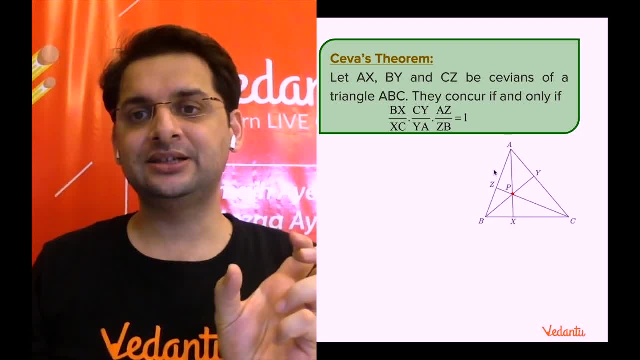 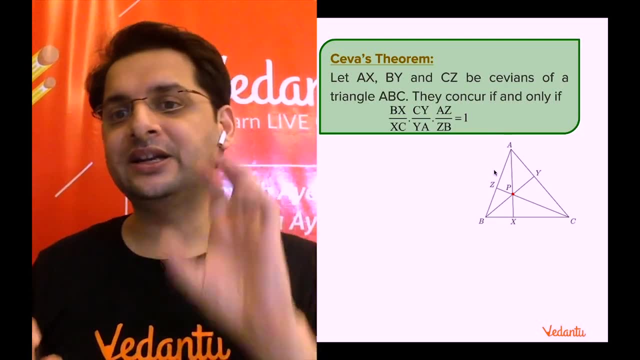 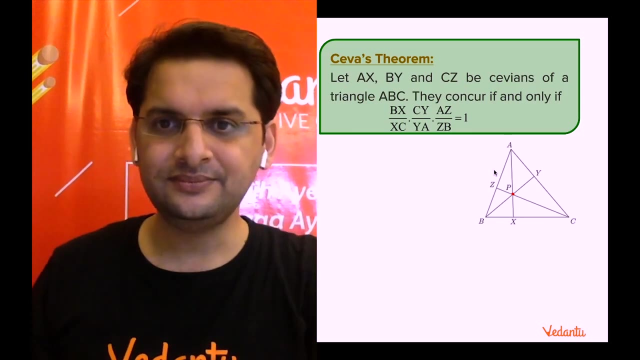 So the ratio of these segments, the product in a cyclic way, is always 1.. So the product of the ratio, So the ratio of these segments of three C wins, taken cyclically in an ordered way, is always 1.. So this is when the three C wins will conquer. 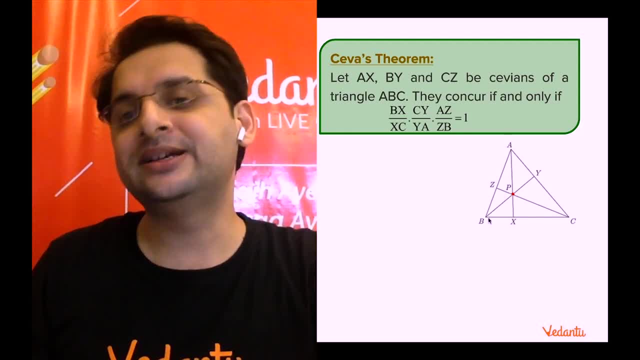 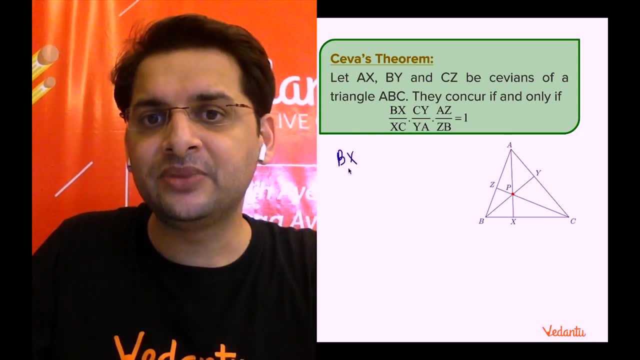 That means they will meet at a common point. And why does this happen? What is the proof? So the proof is: since BX upon XC is involved, So can I say BX upon XC would be what It will be: area of triangle, ABX upon area of triangle. 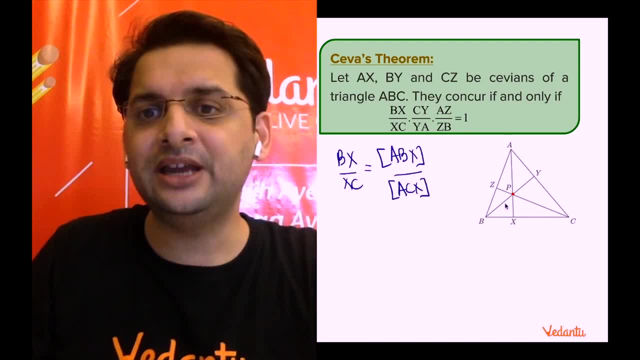 Triangle ACX, because ABX and ACX they have the same vertical height, not AX, but the same vertical height. They have the common point. So half base height, half base height. So the ratio of the bases will be will give me the ratio of the areas. 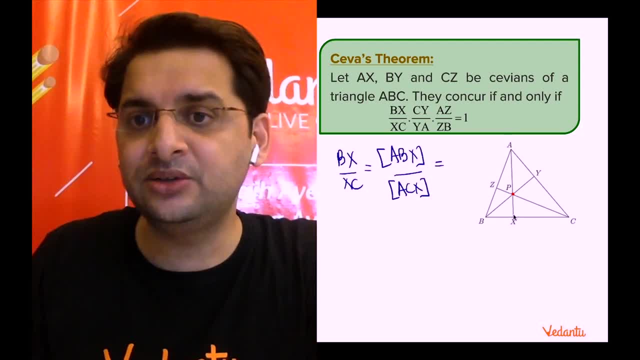 Also can I say, if I talk about BX upon XC, only in triangle, PBX and PXC the same thing can happen. So PBX and PXC, they have the same vertical height. So BX upon X is also equal to triangle area of triangle PBX. 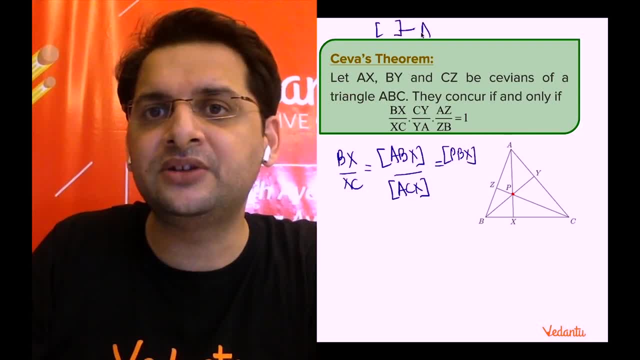 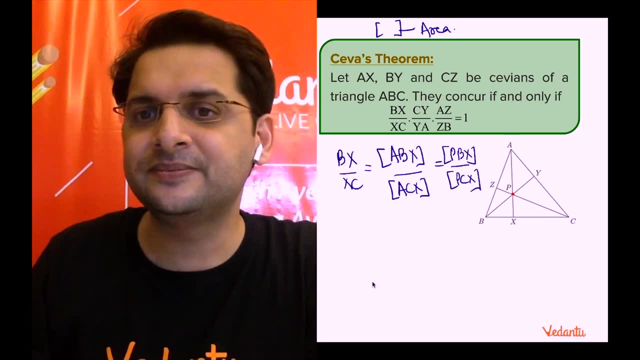 So this means area. This bracket represents area of the triangle Upon area of the triangle, PCX. That is it Also from ratio and proportion. this is, you should be very clear, That A upon B, if it is equal to C upon D, then it is also equal to A minus C upon B minus D. 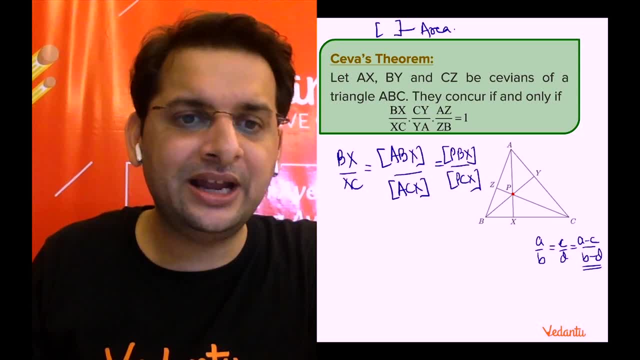 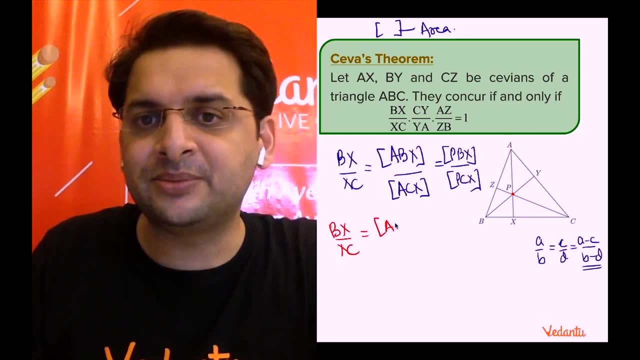 Very important, can be proved very easily. So can I say: BX upon XC is same, as you can subtract these two ratios, So area of triangle ABX minus PBX whole upon area of triangle ACX minus PCX. 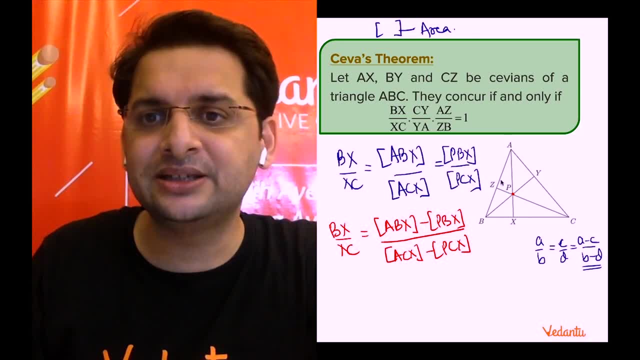 So if we look at the diagram ABX minus PBX, So this gives me ABX minus PBX, gives me this area. So that means BX upon XC is area APB upon. on the right-hand side on the denominator we will get this area APC. 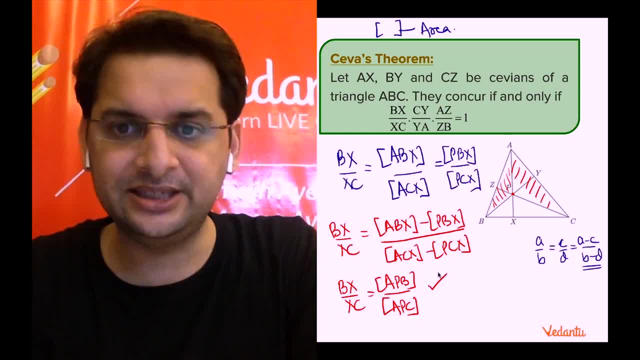 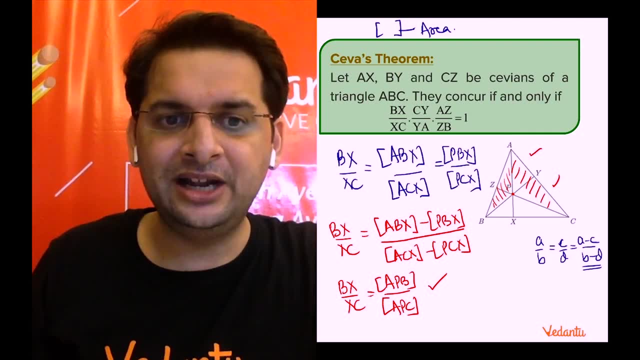 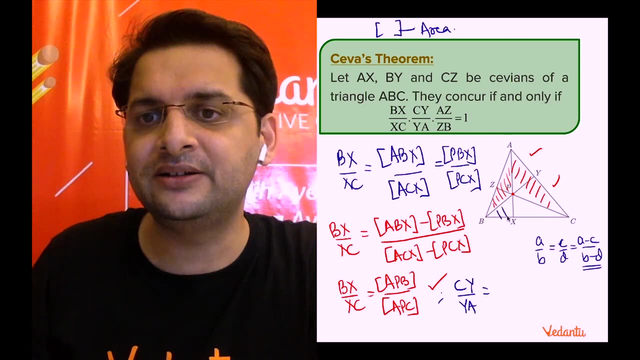 So this is what we have proved: BX upon XC. Likewise, we can also do CY upon AY. So if you can help me with the ratio, similarly, So can I say CY upon AY would give me this area. 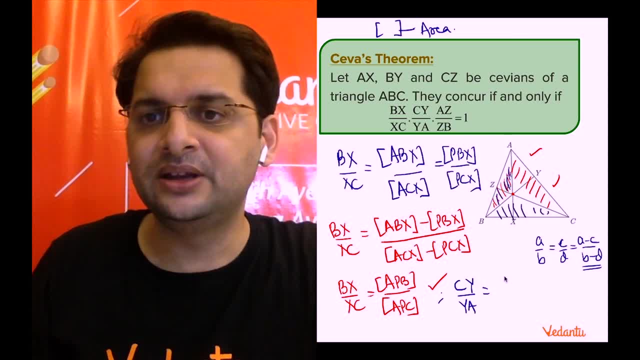 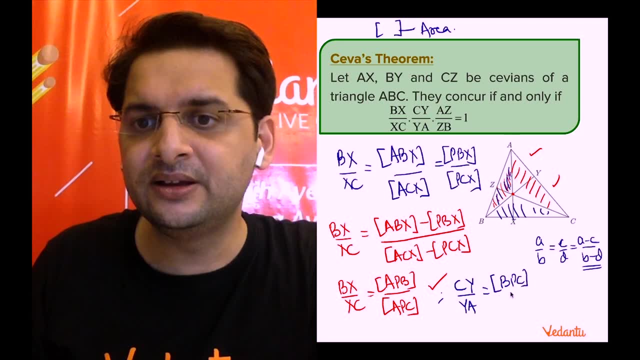 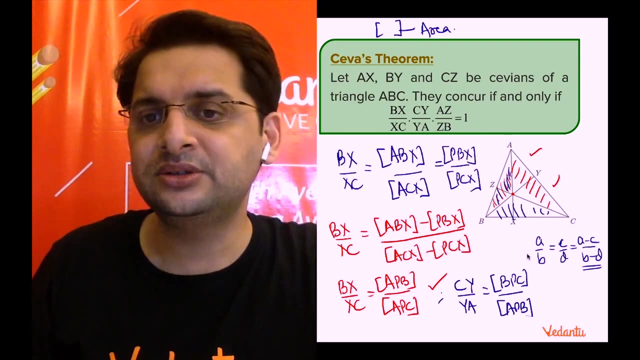 Upon this area in a similar fashion. So this area is area of triangle, area of triangle BPC upon area of triangle APB. And likewise for the third one. we can write the two ratios And if we multiply everything, the right-hand side, if you can see clearly, it will get cancelled out. 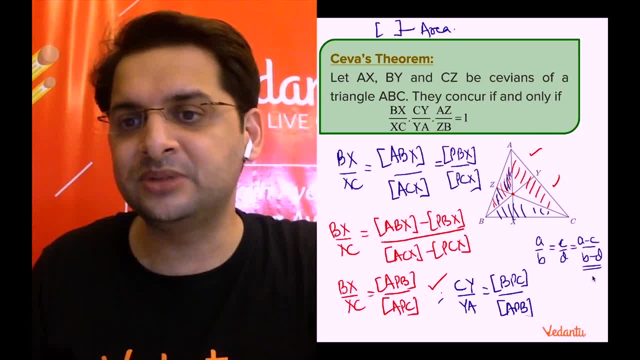 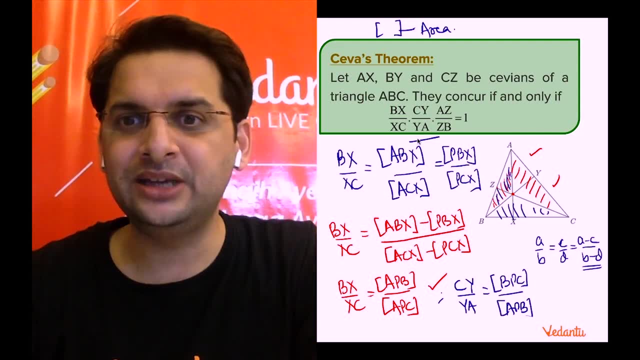 So APB will get cancelled, BPC will get out, cancelled from the third ratio, APC again from the third ratio. So this ratio will come out to be one. I hope this is clear to each and every one. You can have a look at the proof. 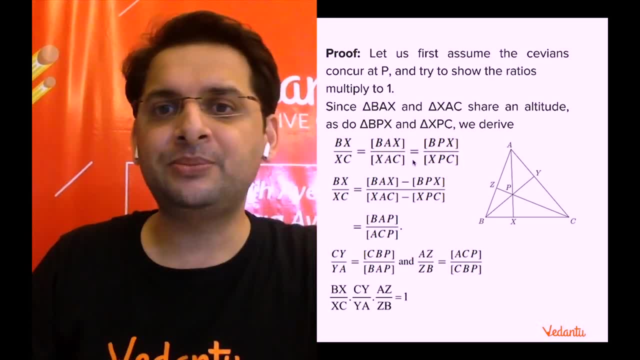 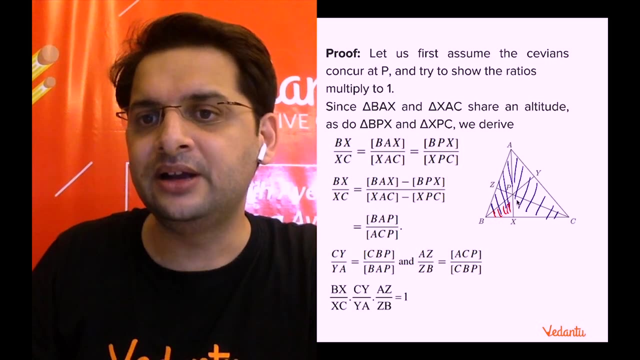 This is how I explain. So BX upon XC is area of triangle BAX upon area of triangle ACX, And this is also equal to area of the triangle BPX, this smaller triangle upon this triangle, because the vertical height is same. 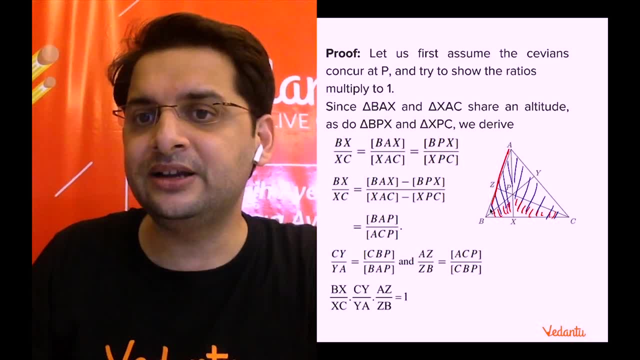 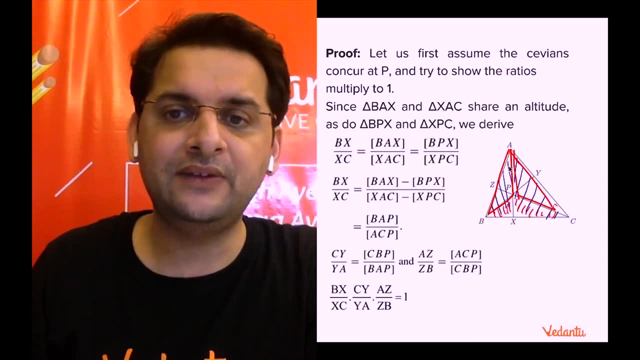 If we subtract these two, so we get. So if we subtract these two, so we get, then we can get BX upon XY, this triangle upon this triangle area, BX upon XYxx, And likewise we can do for CY upon AY, and same thing we can do for AZ upon ZB. 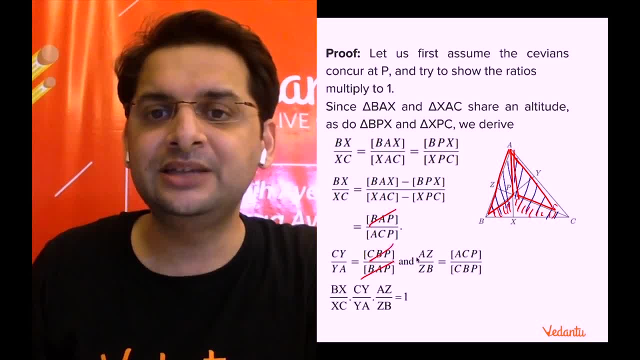 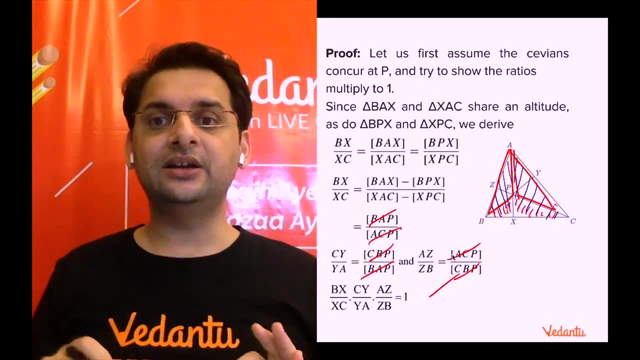 And if I multiply this you can see BAP is getting cancelled out, CBB is cancelled out, ACB is getting cancelled out, So we're getting one. So that means three sevenths of a triangle will meet at a common point. 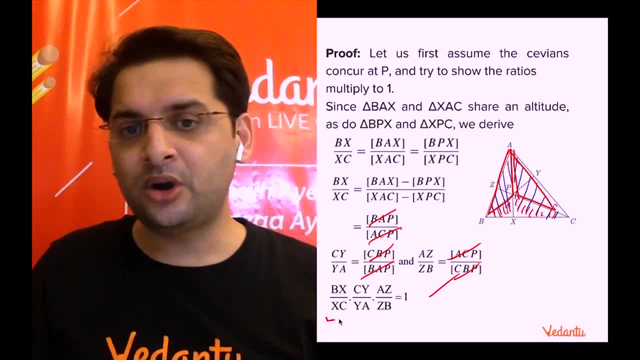 If, and only if, this ratio, so the product of these ratios of the some of these three tenths, should be equal to a Y. So the product of these ratios of the some of these three tenths should be greater of the ratios of the. 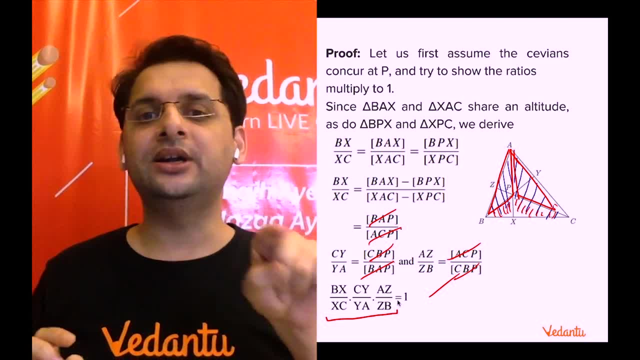 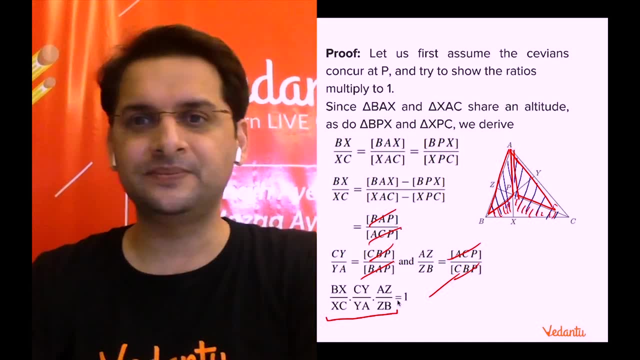 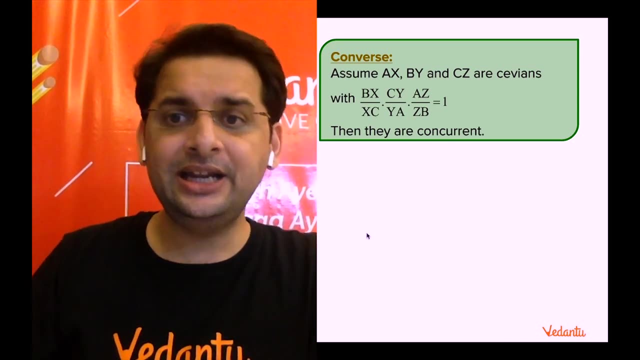 segments of the opposite sides in a cyclic order is 1.. That is it. Take a look. This is so simple a proof and so powerful a theorem. Alright, Now there is a converse also. There is a converse also which says: in a 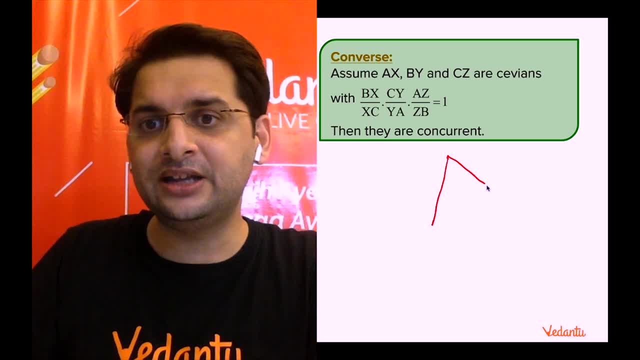 triangle, in a triangle, if there are three C1's- A, B and C. if there are three C1's, let us say this, this and this. so let us say: this is X and Y and Z, so there are three C1's which satisfy this. 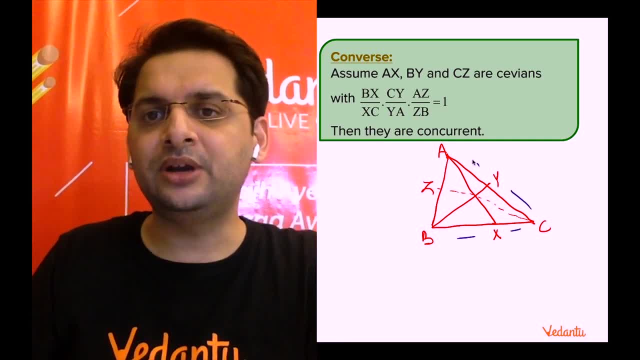 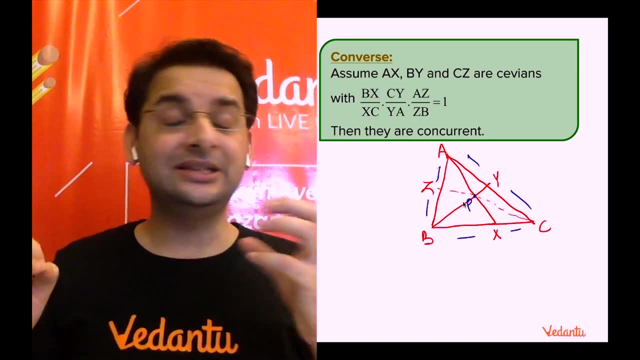 that is, BX upon XC, CY upon AY, AZ upon ZB, is equal to 1.. That means the C1's are concurrent at a point. that means they meet at a common point, P. That is just the converse of what we did. 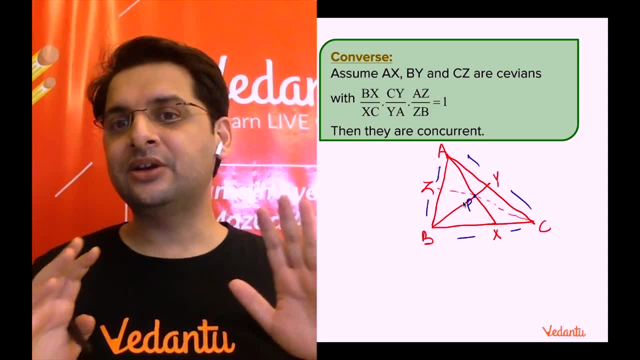 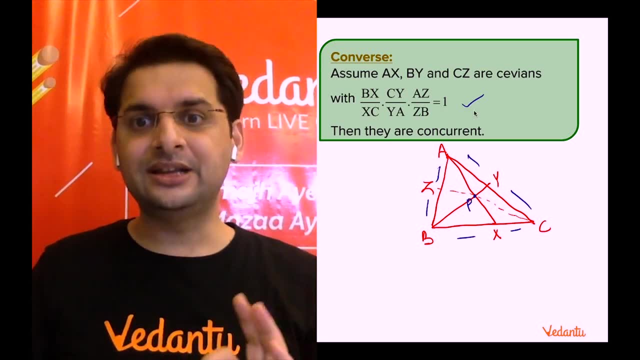 So earlier it was given that they are concurrent, they meet at a common point, and we have to prove this. The converse is, if this holds true, that means the three C1's are concurrent or they meet at a common point, and which is. 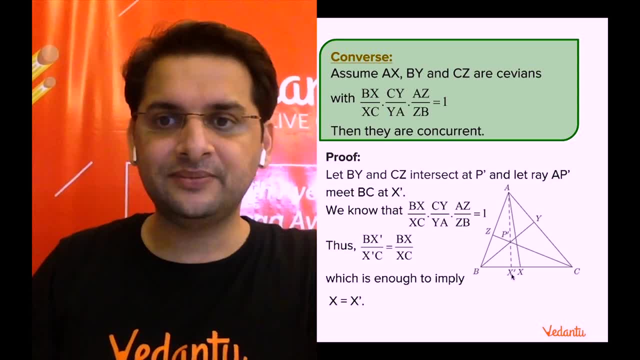 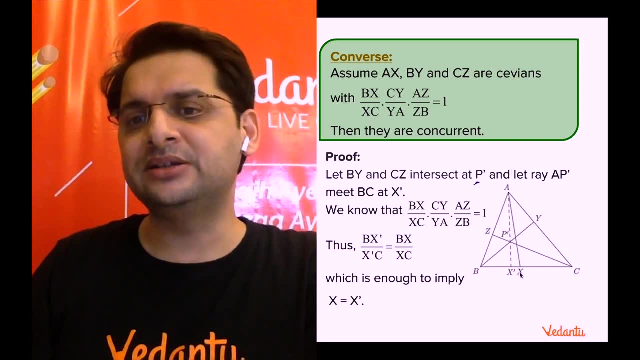 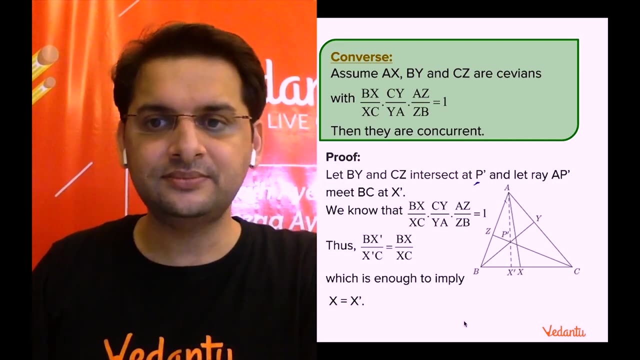 not that difficult to prove. So what we do is, let us say, BY and CZ are two C1's and they meet at P dash and assume that AX does not pass through AX. the third C1 does not pass through this P dash. 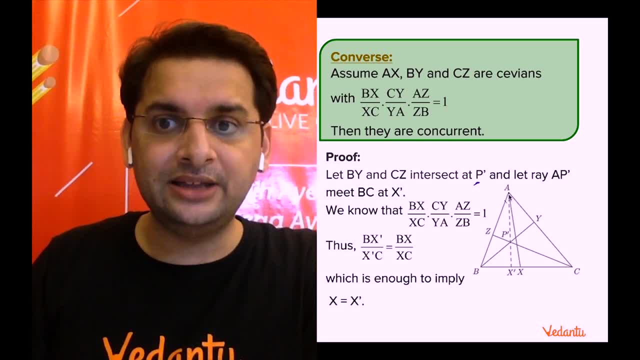 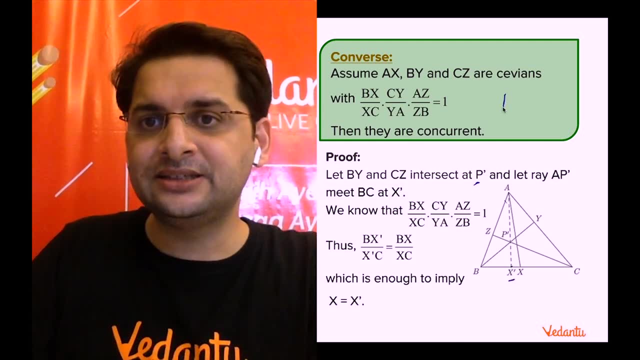 Now let us draw a line joining AP dash and make it intersect at X dash. Now can I say AX dash and BY and CP and CZ are three C1's which are concurrent at a common point, P dash. So we have BX dash upon X dash. 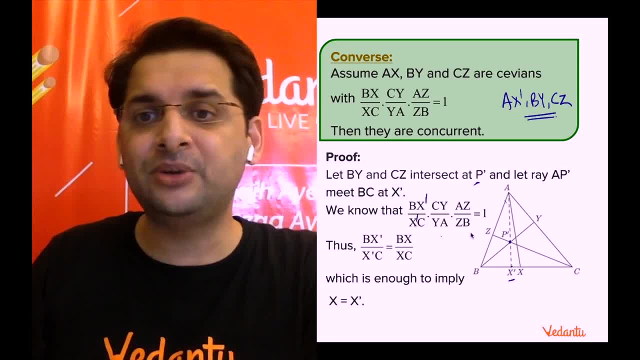 C into CY, upon AY, into AZ, upon ZB, is equal to 1.. And also, we know this is given to us, This is something which is given to us, So if we compare these two, so we will get this. 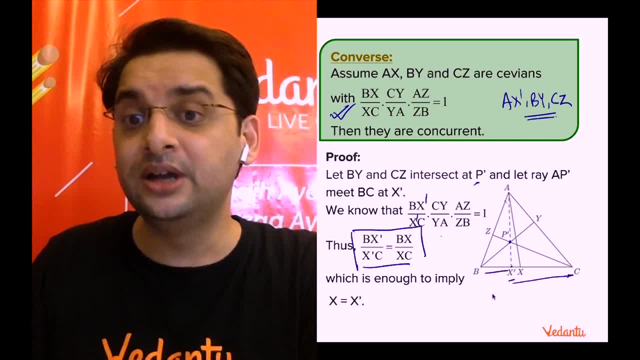 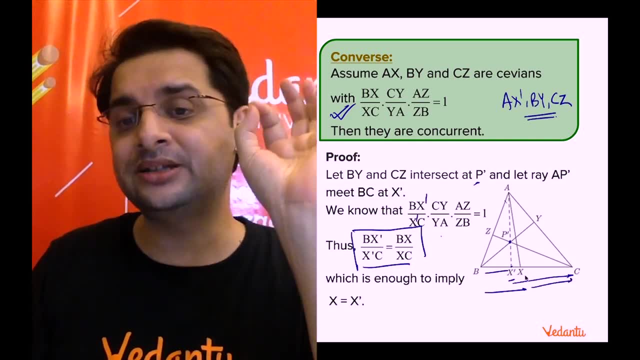 BX dash upon X dash C, So this ratio upon this ratio will be same as this ratio upon this ratio. However, X and X dash are common points or are the points which lie in the interior of PC? And if this holds true, can I say this: 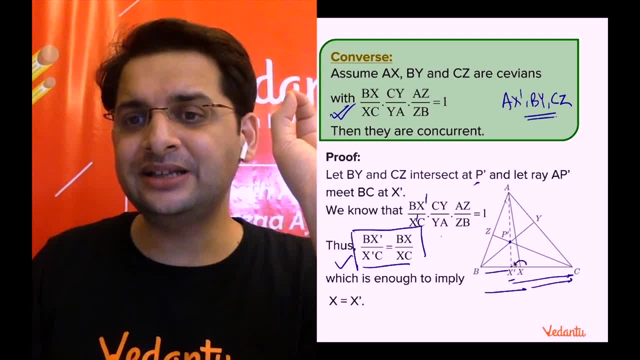 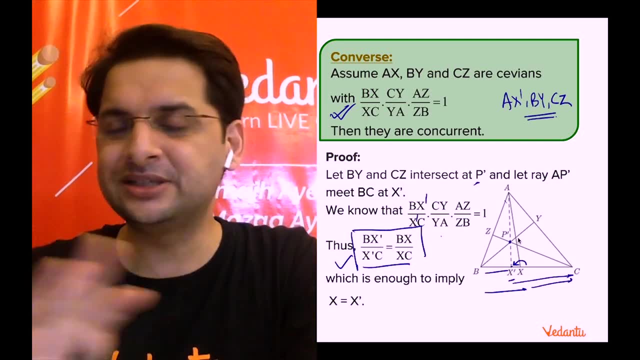 implies that X is same as X dash. So if X is same as X dash, that means that the C1's are concurrent or they meet at a common point, P dash. I hope this is clear. So again, C1 theorem and its converse. 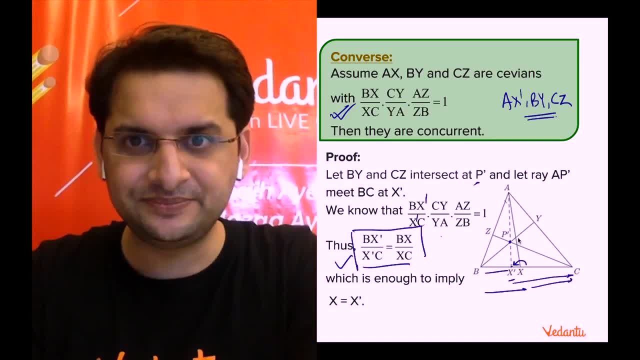 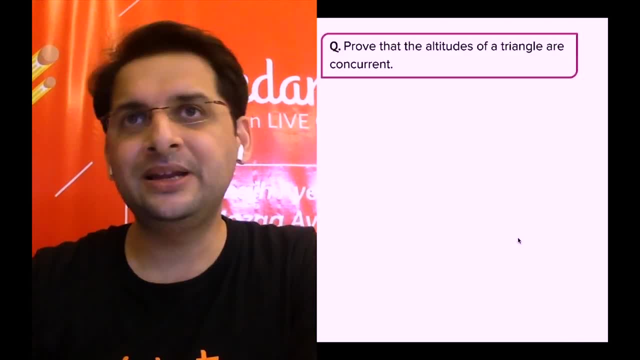 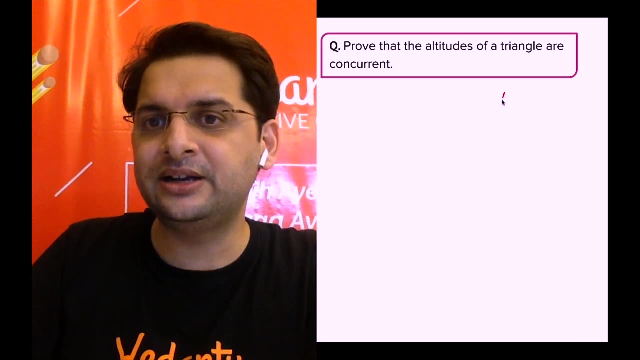 We proved both of them. I hope you all understood this Right. So let us do now a simple application of C1 theorem. The simple application is: we have to prove that the altitudes of a triangle are concurrent, So the three altitudes of a triangle. 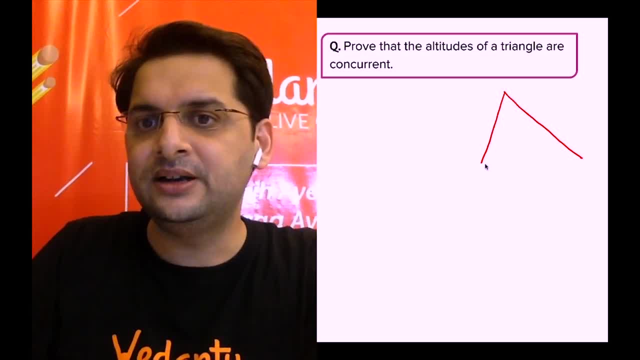 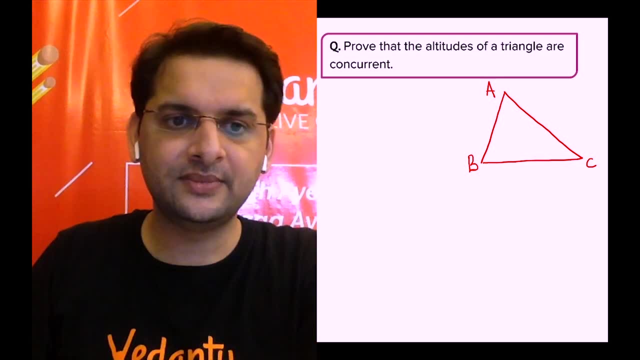 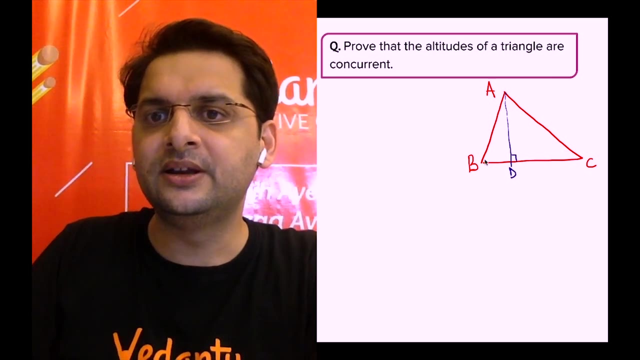 let's just draw a triangle. Let us draw a triangle, So assume that it is an acute angle triangle for the start, And let us draw three altitudes, So we have altitude AD, altitude BE and altitude CF, CF. We all know this. 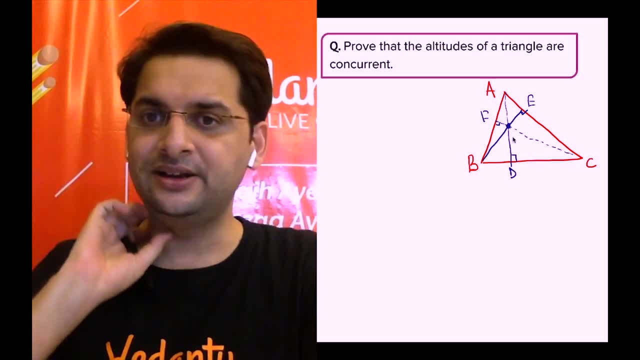 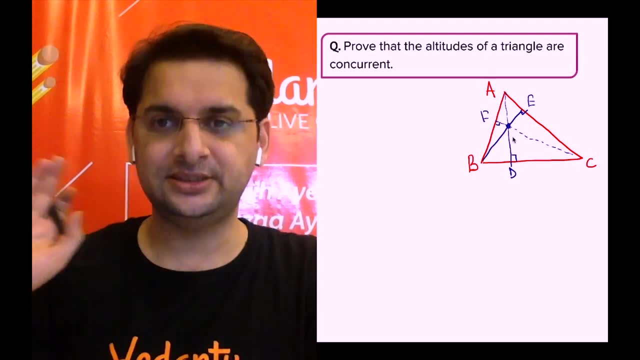 So this is something we have been doing for since the 80s Right, And there are multiple proofs to prove this. So altitudes of a triangle are concurrent. This can be proved in more than one way, But since we have done, 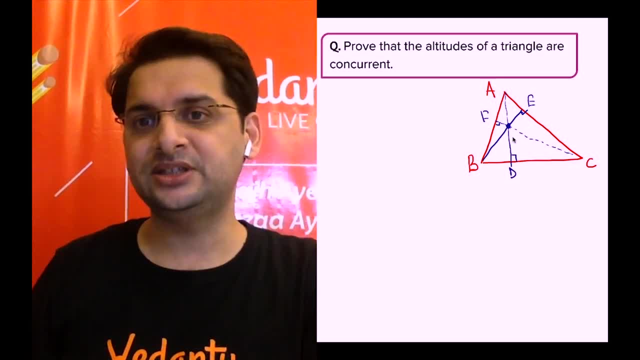 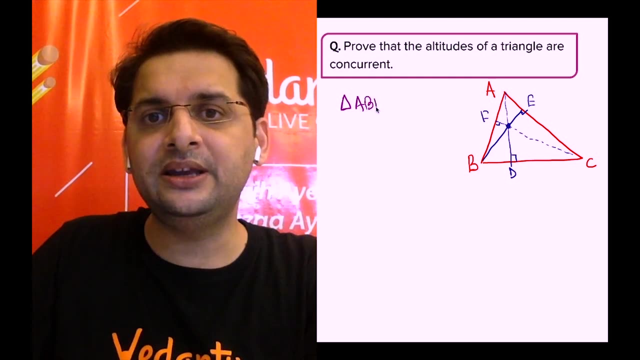 C1 theorem. I am just telling you the simple application of C1 theorem or its converse. Now, how do we prove this? So, how do we prove this? So, if we look at the triangles, A, B, E And triangle, 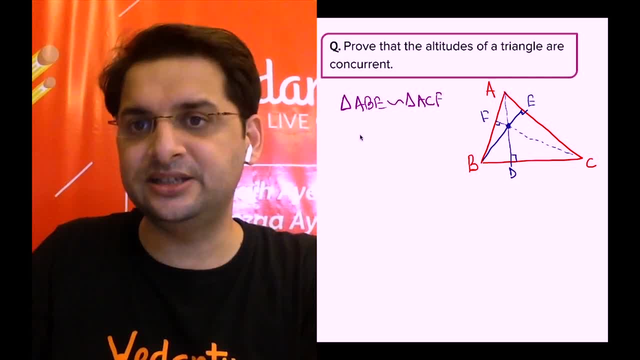 A, C, F. Can I say they are similar in nature, How Angle A is equal to angle A, which is common in both the cases, And angle E is equal to angle F, which is 90 degrees in both the cases. So that means 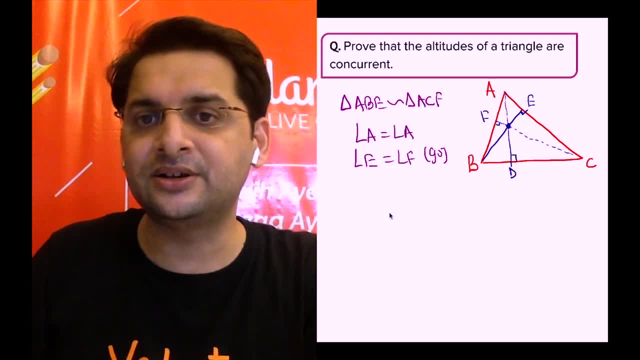 if we compare the ratios and sides opposite to the common angles. So can I say in triangle A, B, E angle opposite to 90 degrees is A, B and A, C, E, A, C, F, the angle opposite to 90. 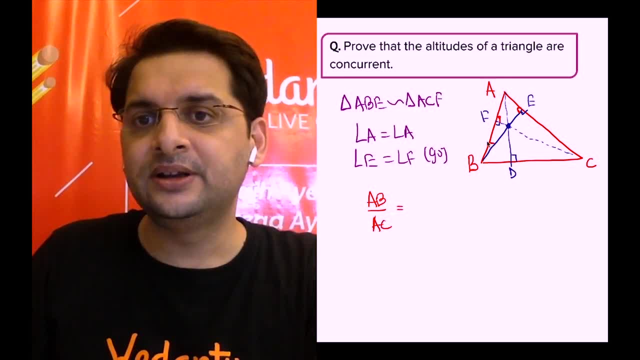 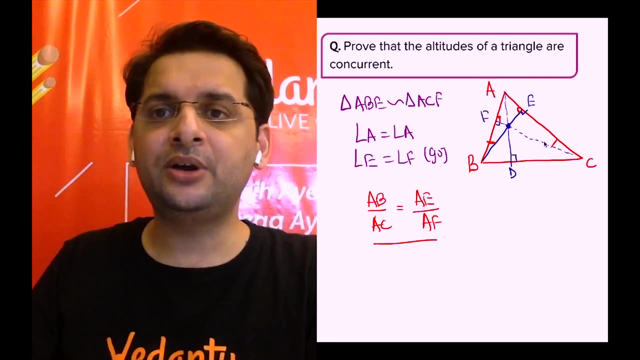 degrees is A- C is equal to common angle. is this? So opposite to B is A E and opposite to C is A F. So simple: A B upon A C is A E upon A F. 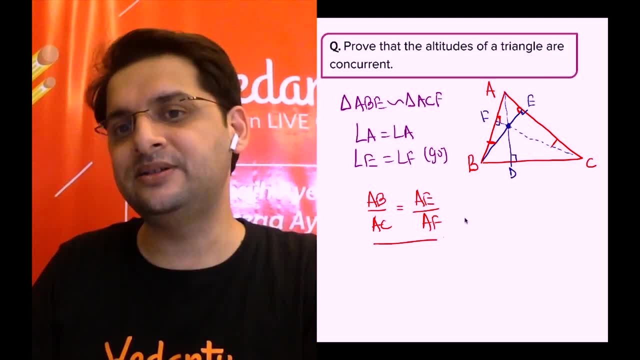 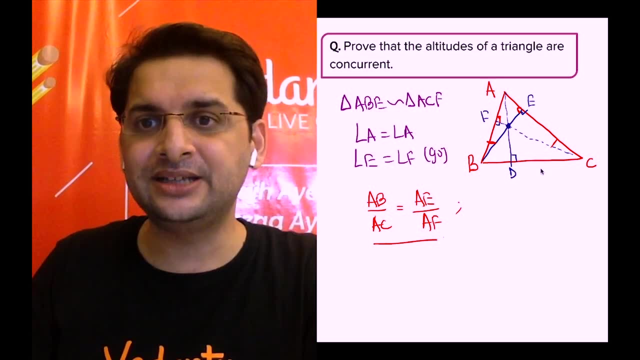 Right, Likewise, likewise for the other two. Remove it cyclically For the others. So can I apply the same in say these two triangles, So triangle B C F and triangle B C E, And likewise. 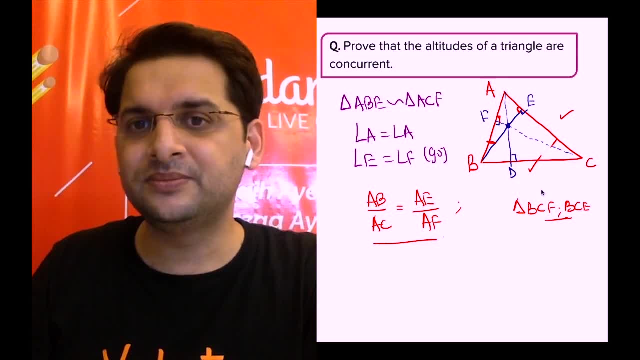 for the third one also. For the third one also Right, So B, sorry, it will be B C E and B C F. Yes, And for the third one also. So if we apply this in a 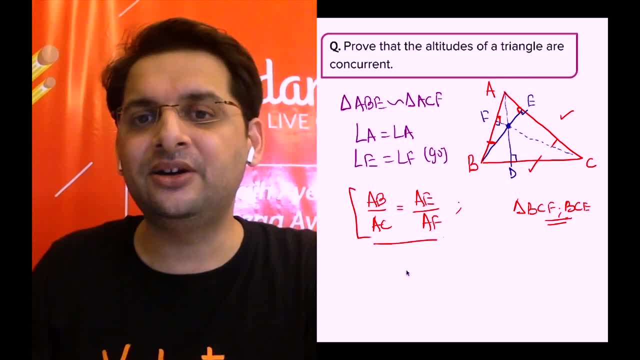 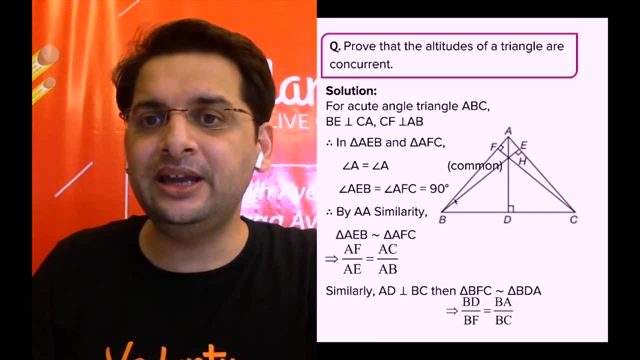 cyclic way. we'll get the sides on one side and these ratios, these small segments, on the other side. So let us see how it goes. So triangle A, E, B is similar to triangle A, C, F, So we 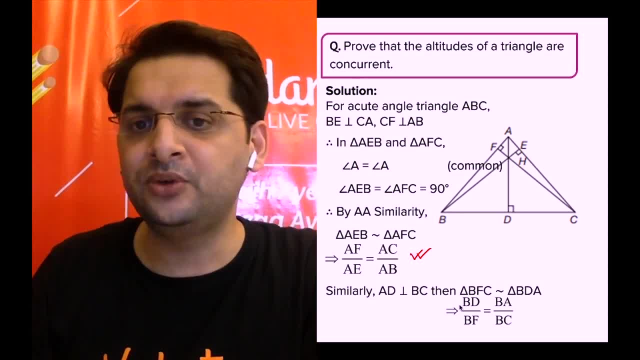 have A F upon A, E is A C upon A B. This is what we proved, Likewise B F C. So B F C is congruent to B D F. It's congruent to B D A. 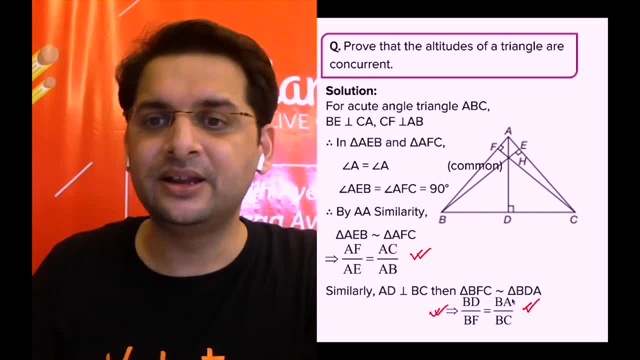 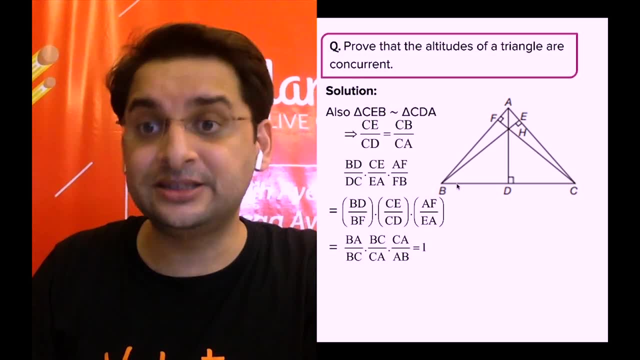 So we have this: B D upon B F is B A upon B C And for the third one, C E. B is similar to, is similar to- I think I said congruent before- is similar to. 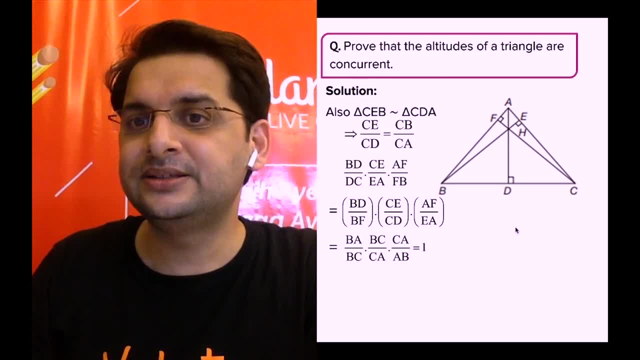 C D A, C D A, Because angle C is common and two angles are 90 degrees. So that means C E upon C D, is C B upon C A. So if we multiply all the three ratios, 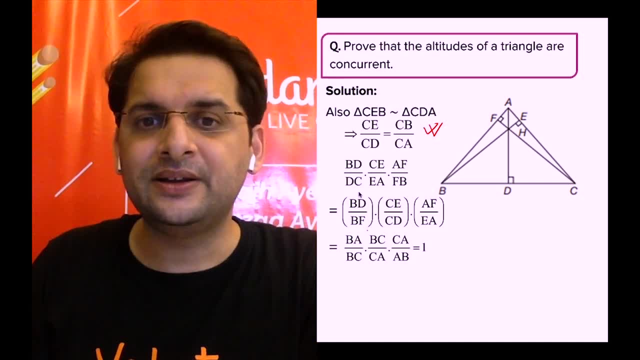 If we multiply them, So B D upon B F, Sorry, B D upon D C, B D upon D, C is C, E upon E, A is A, F upon F, B And right hand side. 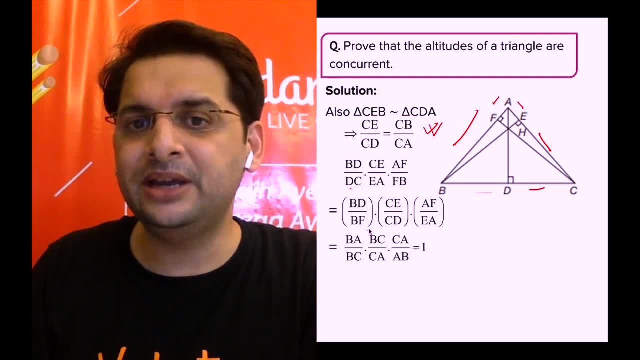 we get all the sides: B, D upon B, F, C, E upon C, D, A, F upon E, A, If we rearrange them. And right hand side we have all the sides. So C, A gets cancelled, A, B gets cancelled. 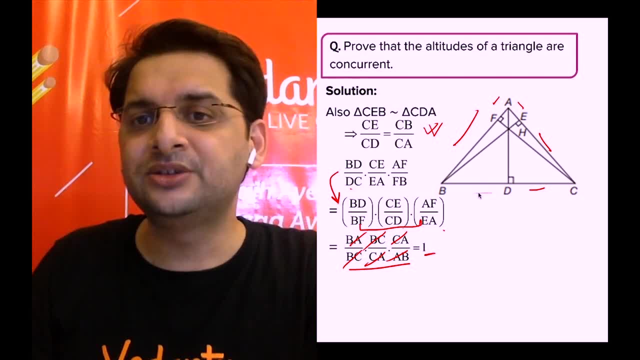 B, C gets cancelled And this comes out to be one. So B, D upon B, F, C, E upon C, D, E, F upon E. A is equal to one, And this can be rearranged at this. 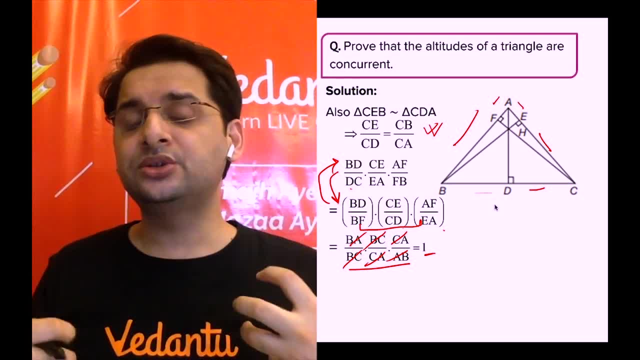 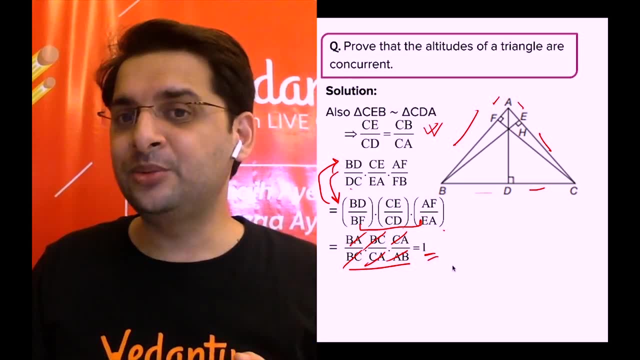 So that means the product of the ratios of the segments of the opposite sides, in a cyclic way, is coming out to be one. And if this comes out to be one, that means that these events, which in this case is the altitudes, are.